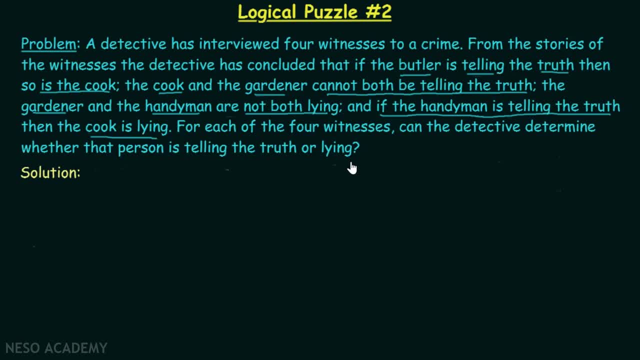 You have four witnesses and their statements. On the basis of the statements, you need to determine whether they are telling the truth or they are lying. Let's start solving this logical puzzle, And the idea is to solve this puzzle using propositional logic. 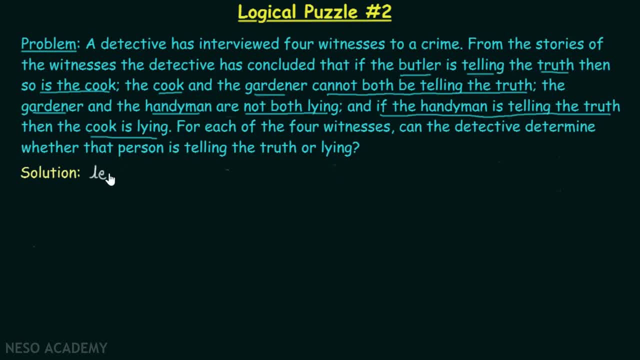 Let's see how we can do that. Let b be a propositional variable which is equal to butler is telling the truth, Right. Let c be a propositional variable that cook is telling the truth. Let g be a propositional variable representing that. 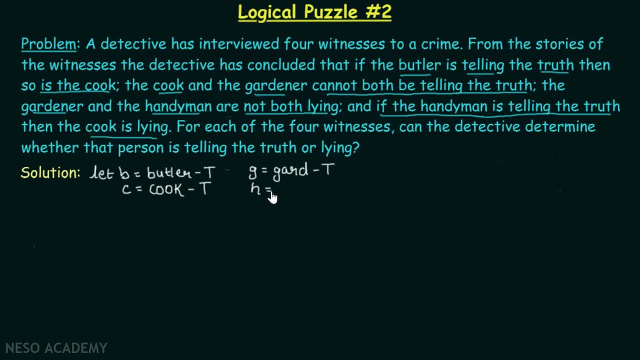 gardener is telling the truth. And let h be a propositional variable which represents that handyman is telling the truth. Okay, Now, as b is butler is telling the truth, let's say: not b represents butler is lying, Not c represents cook is lying. 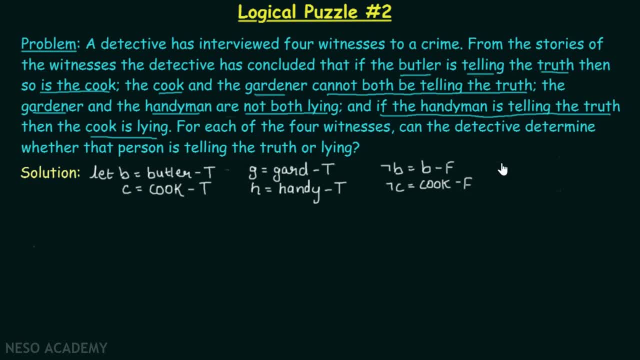 Not g represents that gardener is lying And not h represents handyman is lying. Now let's consider these statements one by one. Let's consider the first statement. If the butler is telling the truth, then so is the cook. This statement is of the form. 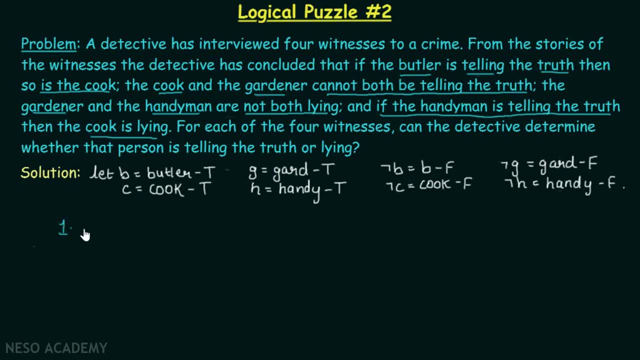 if p, then q. Therefore, this is equivalent to b implies c, Right? If butler is telling the truth, then cook is also telling the truth. Right Now let's consider the second statement. The cook and the gardener cannot both be telling the truth. 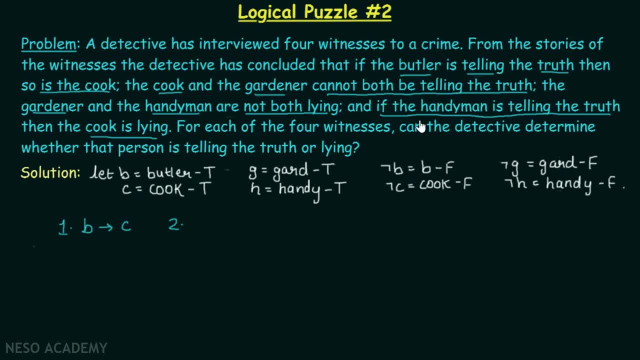 How do we represent this in propositional logic? Simple: Let's say: cook and gardener both are telling the truth. This statement represents that cook and gardener both are telling the truth. Now, if we place a not in front of this particular expression, 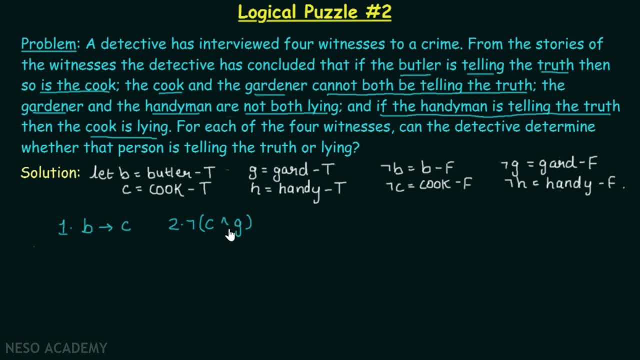 then this expression is equivalent to both cook and the gardener are lying, Isn't that so? So this is equivalent to not c or not g. Right, Let's consider the third statement. The gardener and the handyman are not both lying. 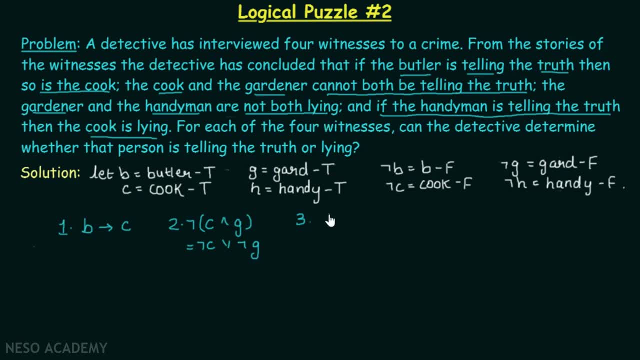 Let's represent this statement in propositional logic. Not g and not h simply means that both gardener and handyman are lying. Now, if you want to represent that both gardener and handyman are not lying, then simply put a not in front of this expression. 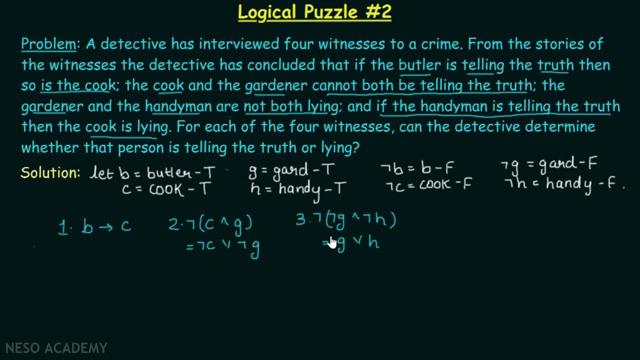 This becomes g or h. Because of this, not this conjunction will become disjunction, As in this case. also, because of not, conjunction becomes disjunction. Let's consider the fourth statement. If the handyman is telling the truth, then the cook is lying. 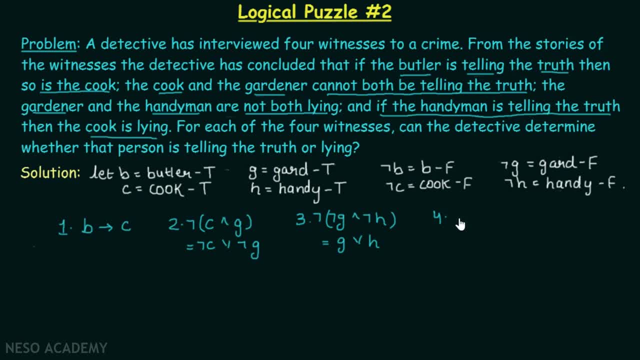 Now, this is also of the form: if p, then q. Right, This is equivalent to h implies, not c. If handyman is telling the truth, then cook is lying. Simple. Now, how can we determine that each of these four witnesses are telling the truth? 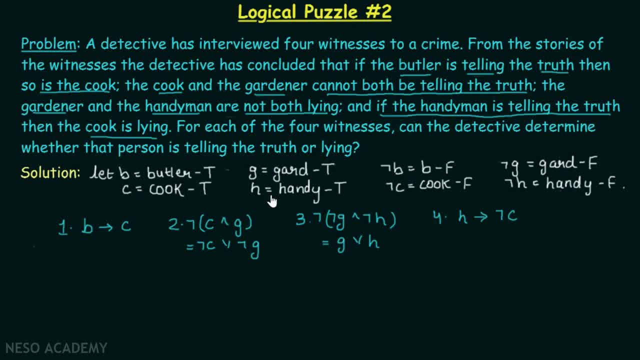 or they are lying. Let's take one assumption, And with the help of that assumption, we then come to some conclusion. If that conclusion is satisfactory, then we would be able to determine whether each of these witnesses are telling the truth or they are lying. 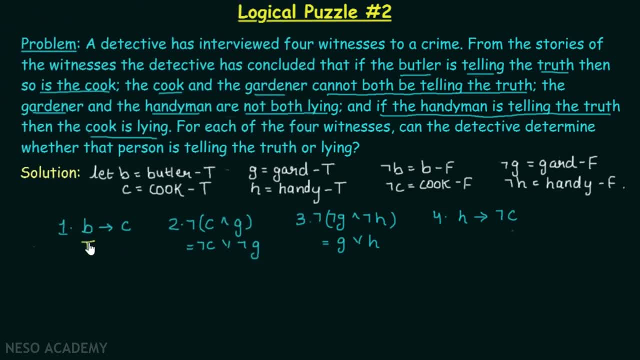 Let's say b is true, And if b is true then c has to be true Because of implication. Now, if c is true, then not c is false And if not c is false according to the disjunction, this has to be true. 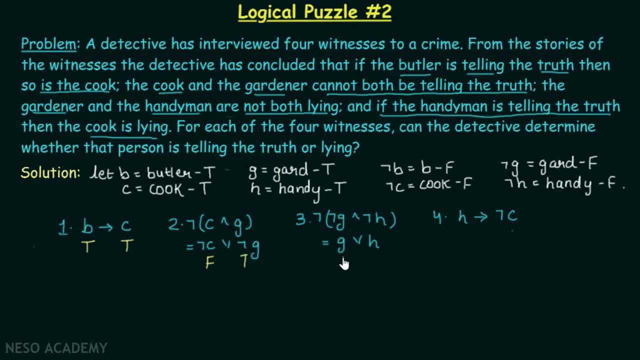 Right, And if not g is true, then this has to be false. And if this is false, then this has to be true. Now, if h is true, then this cannot be false Right. But, as we know, not c is false. 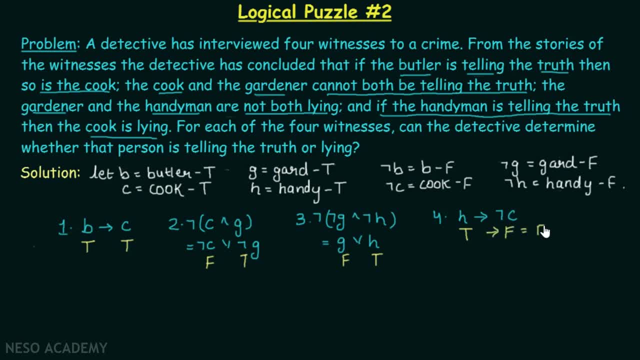 Therefore, the final implication becomes false, As we are successful in making this particular expression true, this one true, this one true, but we would not be able to make this expression true. Therefore, this is the contradiction, And hence b cannot be true. 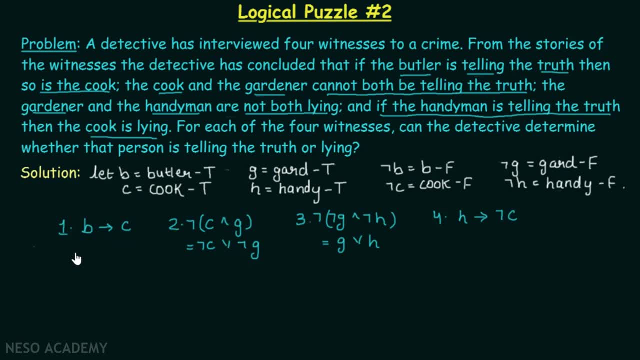 Right Now. let's take b- false. If b is false, then we know that c can be true or c can be false. Let's take c- true. If c is true, then not c is false, And if not, c is false. 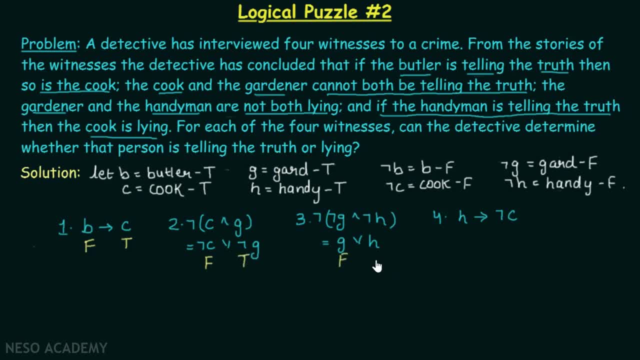 this has to be true. Similarly, this is false and this one will be true, And if h is true and not c is false, the final implication will become false, Which is again a contradiction, And hence we can conclude that c cannot be true as well. 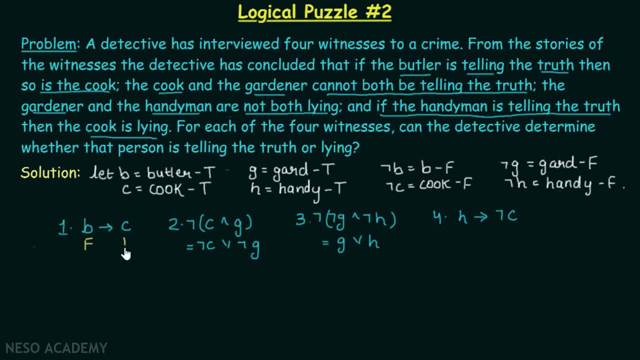 Okay, Now let's take c false. If c is false, then not c will be true, And we know that if not c is true, not g can be true or not g can be false. Let's take not g true If not g is true. 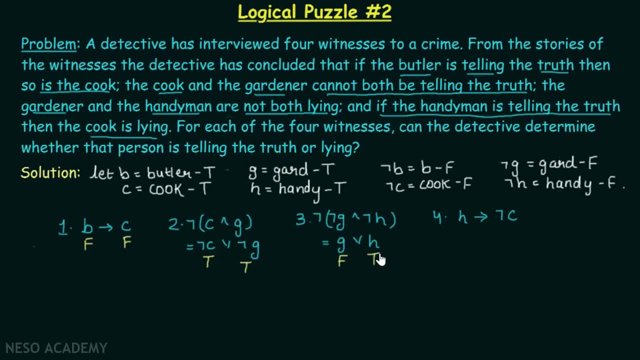 then g becomes false, And if g is false, then h has to be true. Now, as h is true, then, as we know, not c is also true, and true implies true is true. This expression is true. this one is also true. 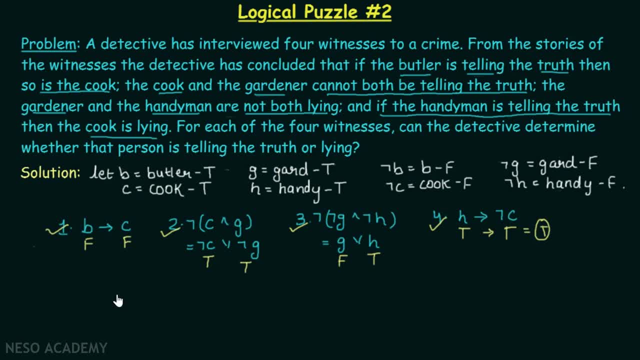 this one is also true, and this one is also true. Therefore, we come to this conclusion that b is false, c is false, g is false and h is true. But we cannot stop here. We have to go further, As we know that we have chosen. 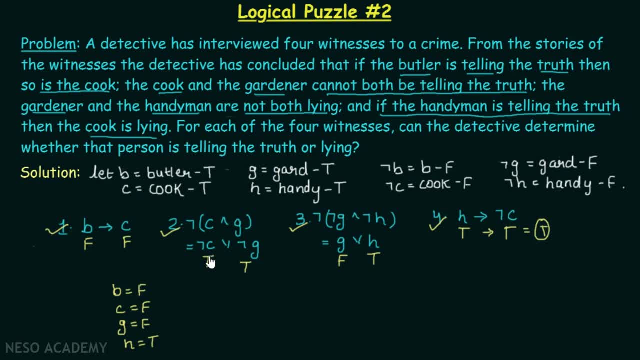 just one truth value of not g. But, as we know, if not g is true, we can choose some other truth value of not g We can take false. also, Let's take not g false. If not g is false, then g would be true. 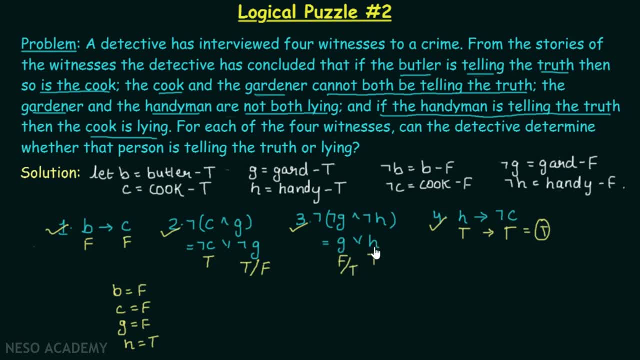 Right. And if g is true, we know that h can be true or h can be false. Right, Let's take h true, and in that particular case the combinations are still satisfied. Therefore, the another combination would be that b is false.